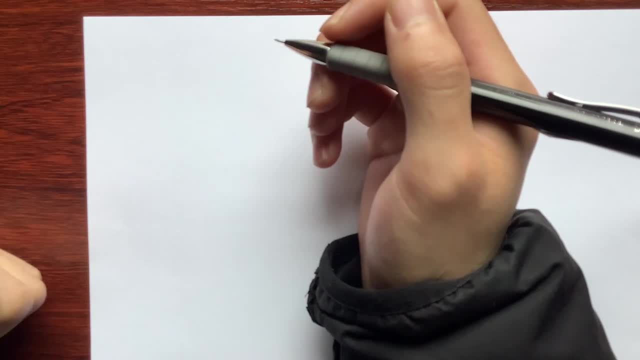 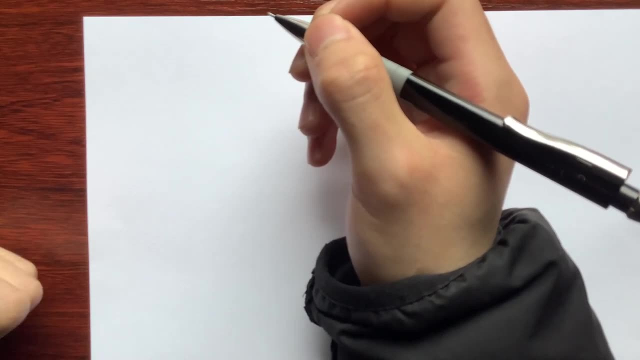 particle does not change with time. Mathematically, a stationary state is a solution of the time-independent Schrodinger equation, which describes the behavior of a quantum mechanical system in the absence of external forces. A stationary state is characterized by the specific energy. 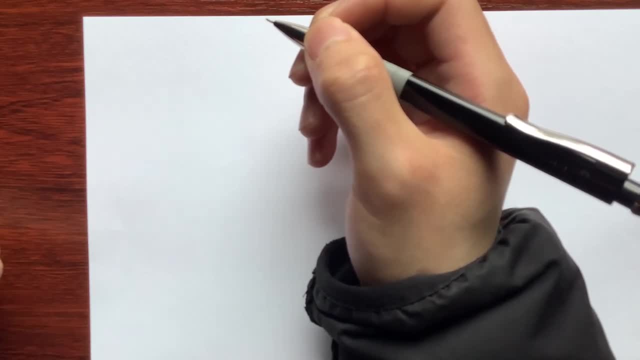 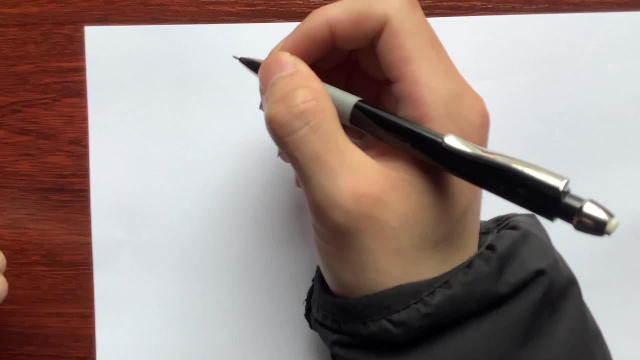 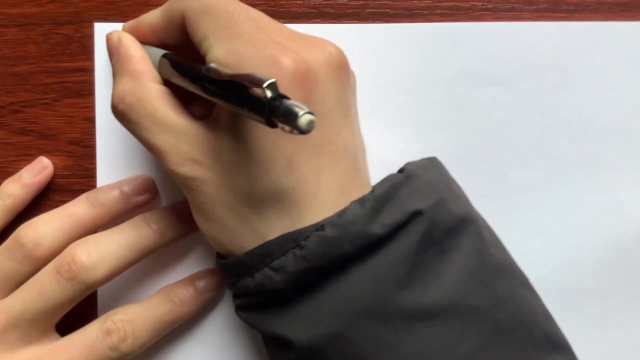 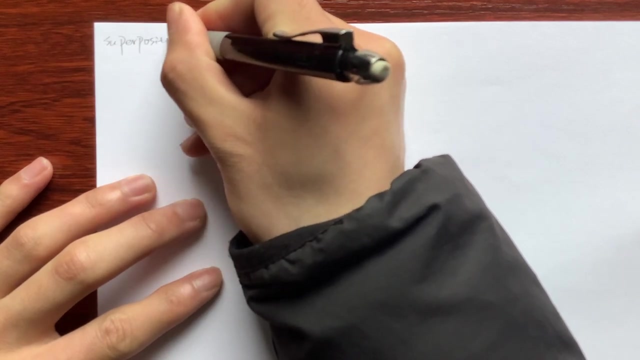 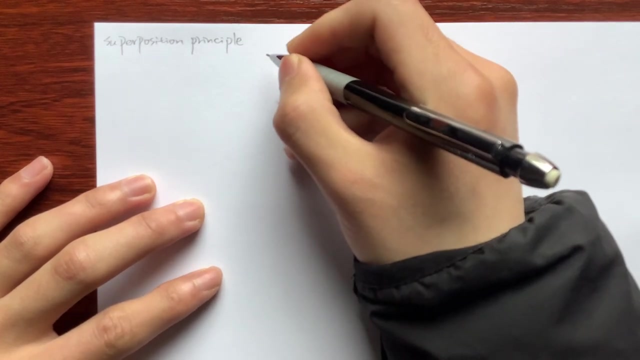 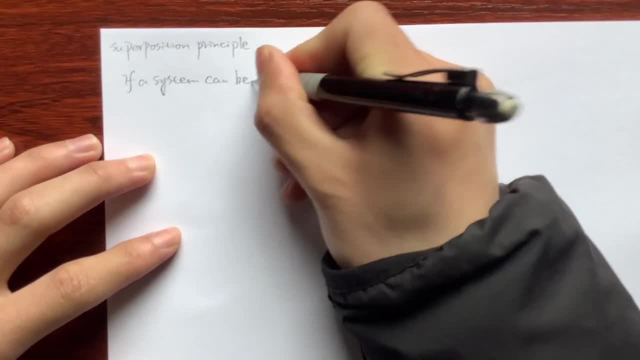 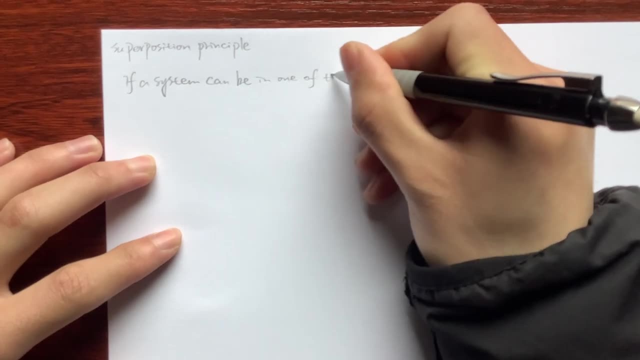 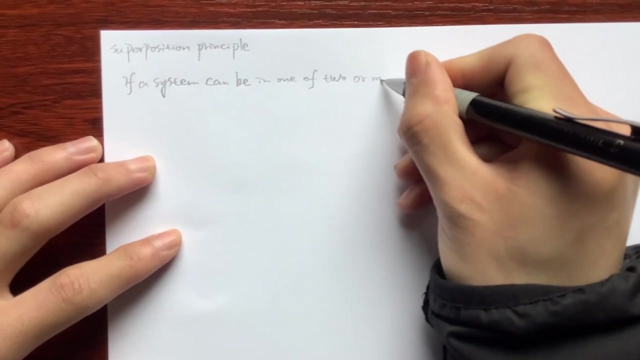 So connection is the pre mall Head, So connection is the pre mall Head. So real person and trust mechanism. So real person and trust mechanism. If ourORE cannot know DOT, If it can sense, DO NOT KNOW DOPS. 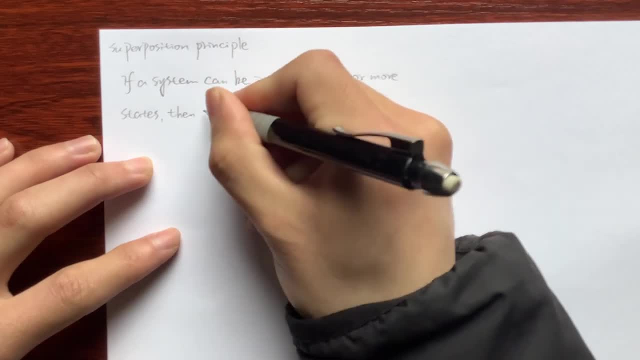 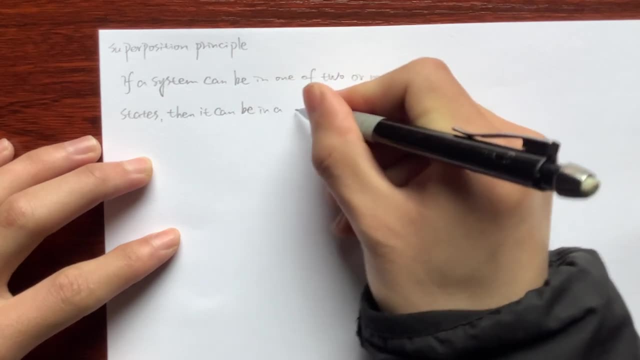 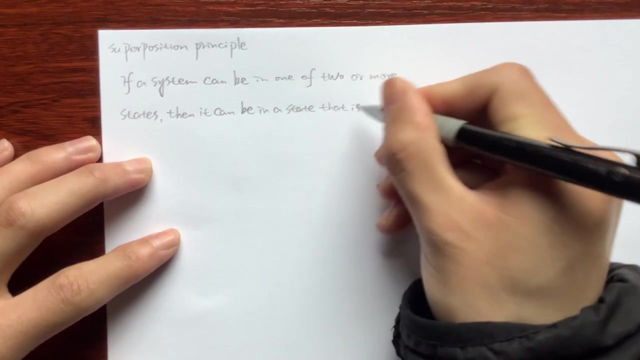 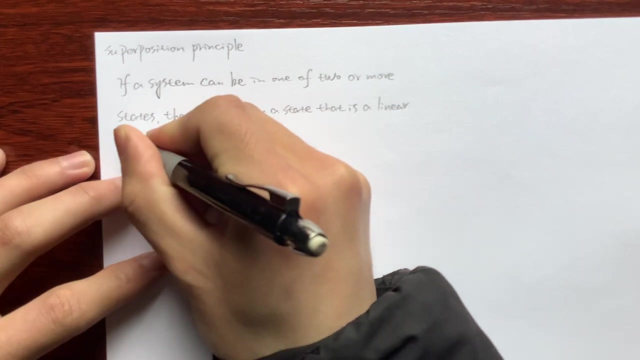 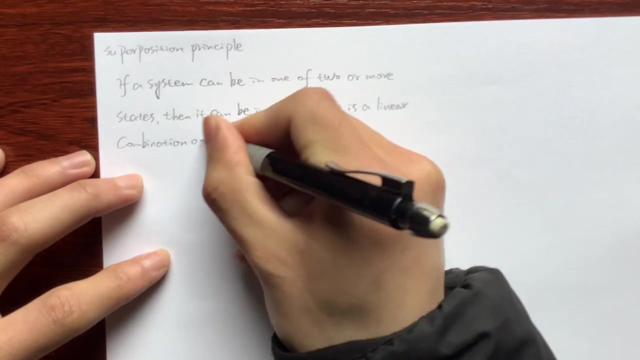 If it has doubt, DO NOT KNOW DOPS. If its a small little spot on earth, INSURNAL IDEA. IF it has doubt, DO NOT KNOW DOPS. IF its a small little spot on earth, INSURNAL IDEA. Thank you. 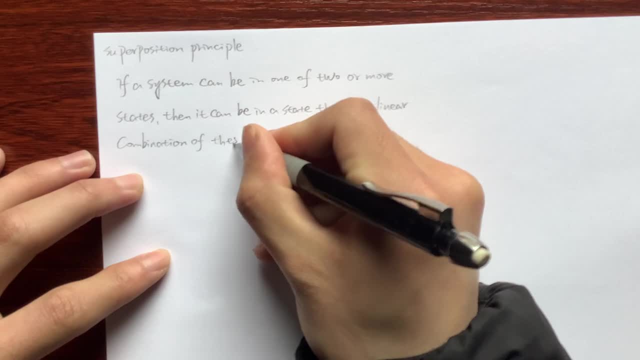 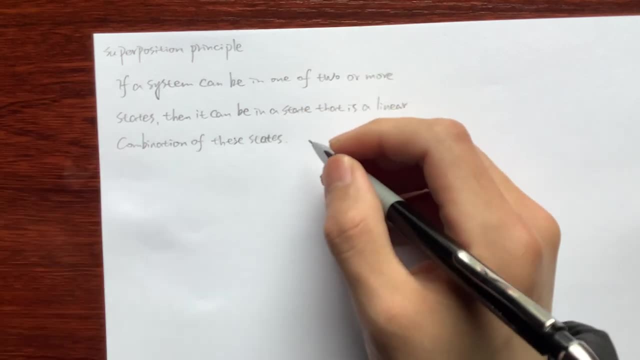 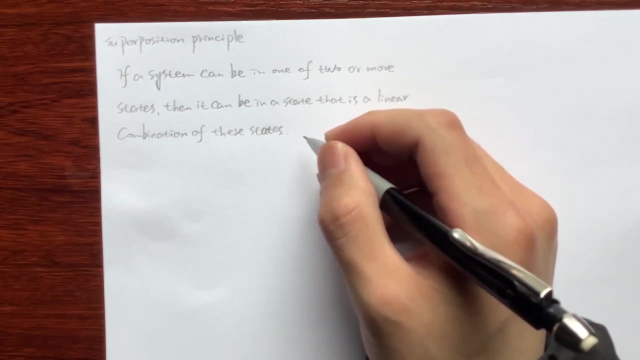 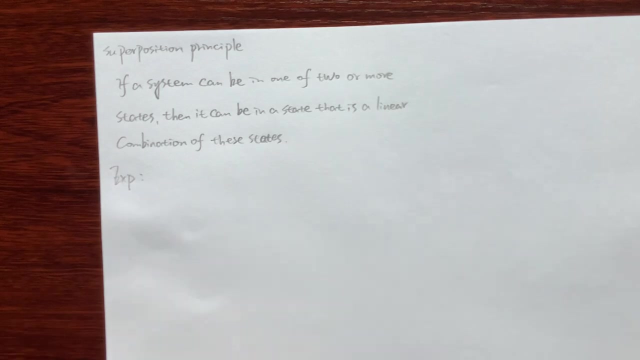 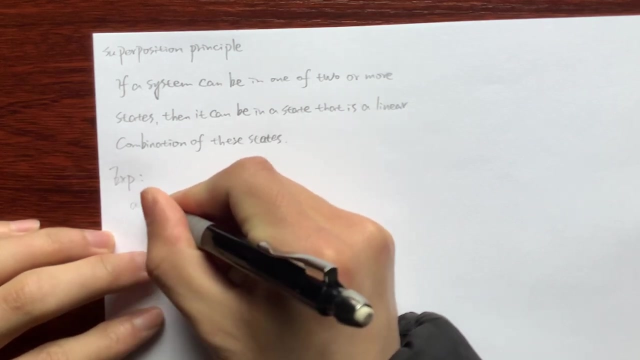 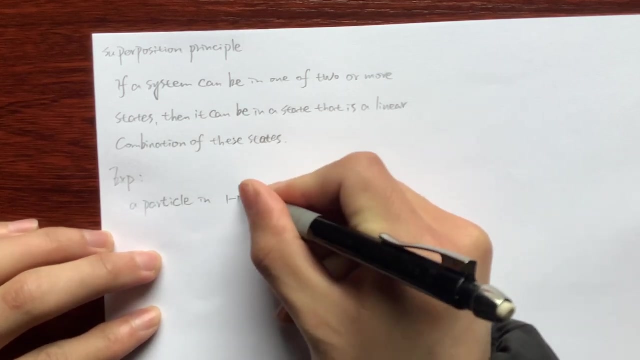 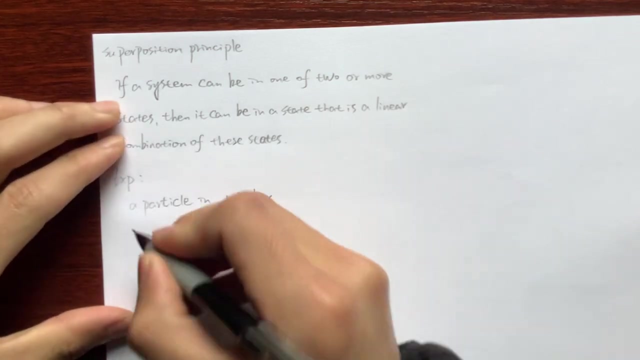 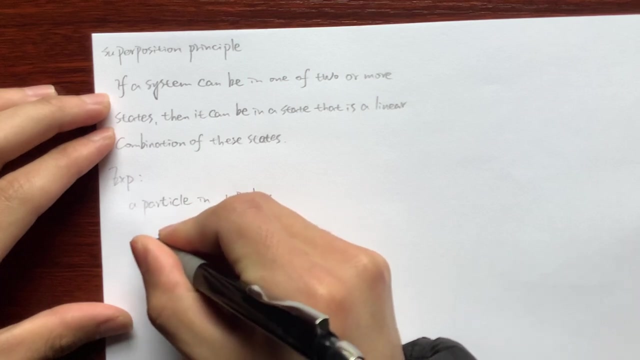 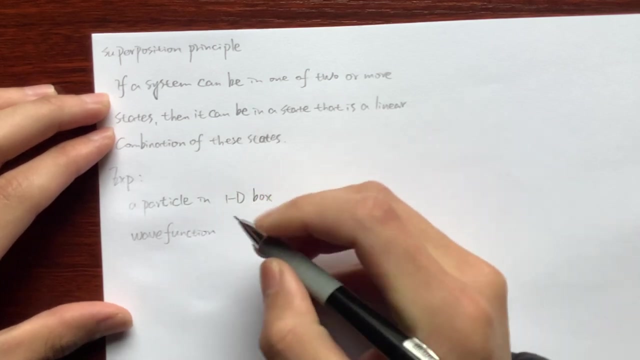 Now let's discuss the example. Let's consider a particle in a one-dimensional box. The wave function for the particle in the ground state is n equals to 1.. Now let's consider a wave function. The wave function for the particle in the ground state is n equals to 1.. 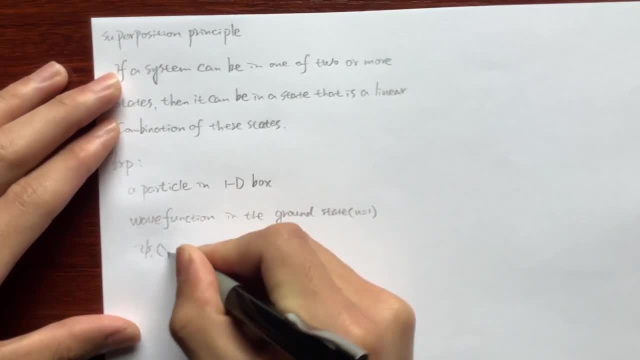 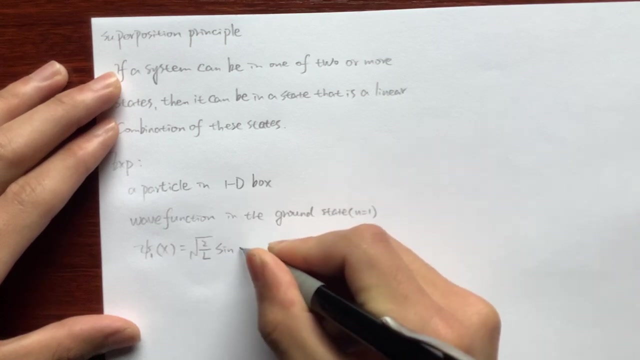 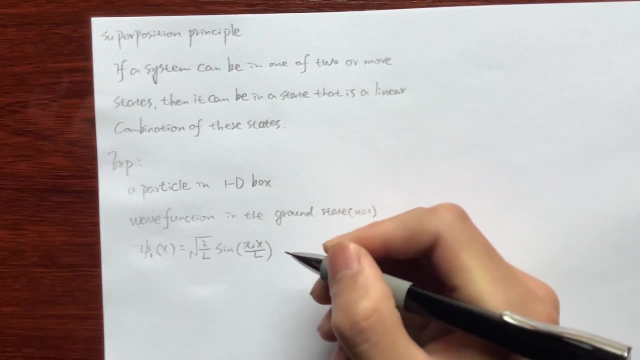 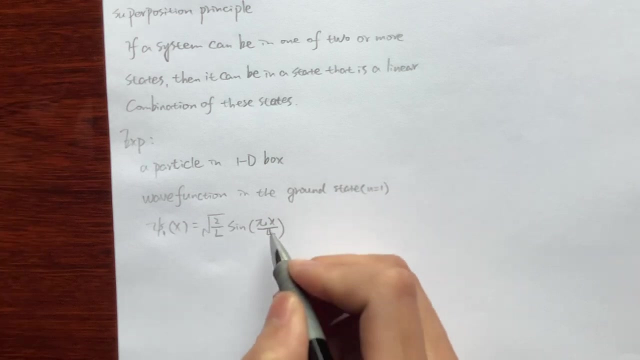 And it's given as phi sub 1 of x equals to square root of 2 over L times sine of pi x over L. L in here is the length of the box and x is the position of the particle, The wave function for the particle in the first excited state. 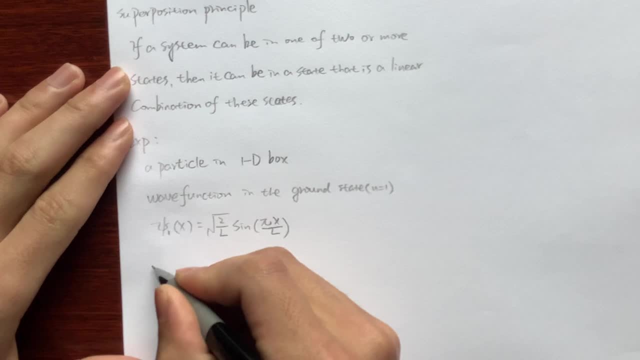 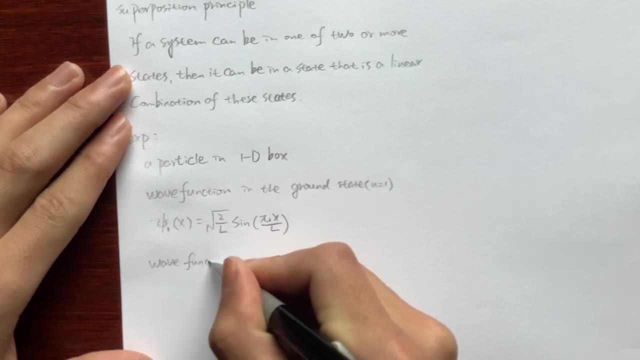 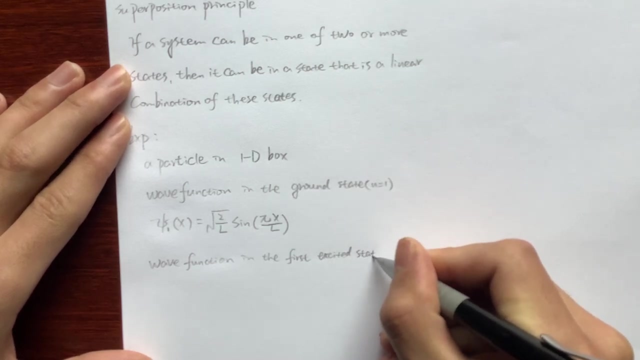 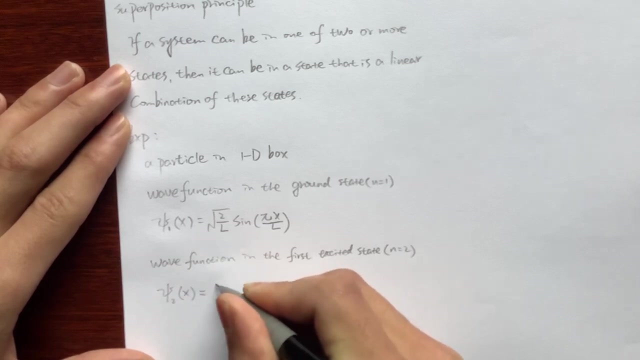 is n equals to 2.. So let's write it down: Wave function in the first excited state is n equals to 2. And it's given by square root of 2 over L times sine of 2, pi x over L. 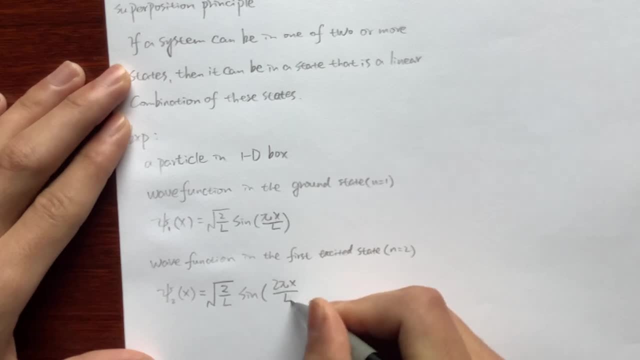 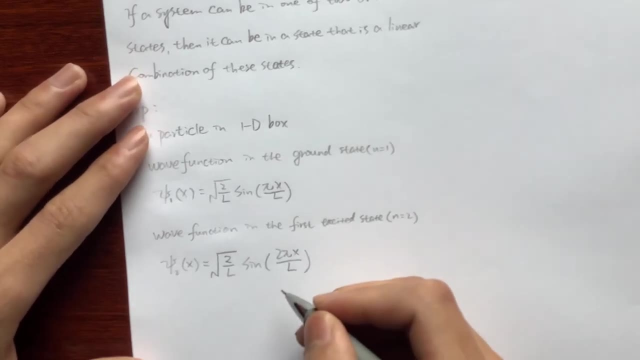 square root of 2 over L times sine of 2 pi x over L. square root of 2 over L times sine of 2 pi x over L. Our кв is now n. sine of n equals to n. Now we can take a look at the你就 N. 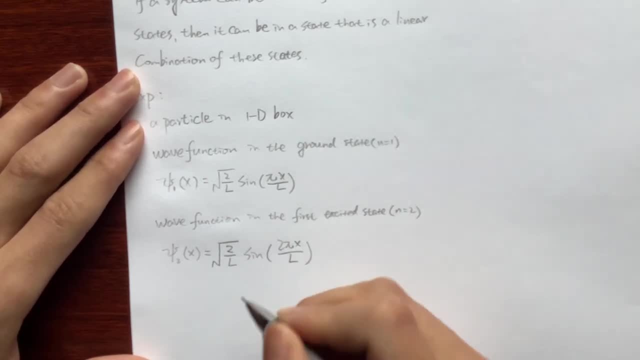 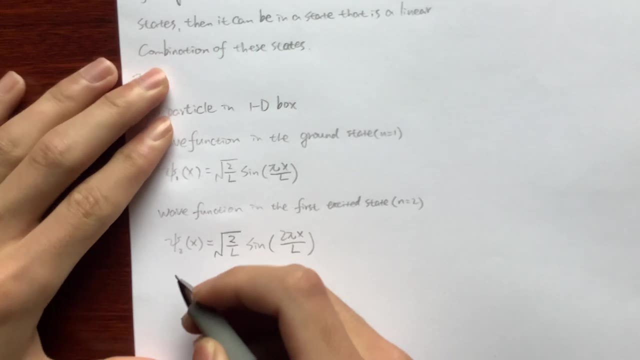 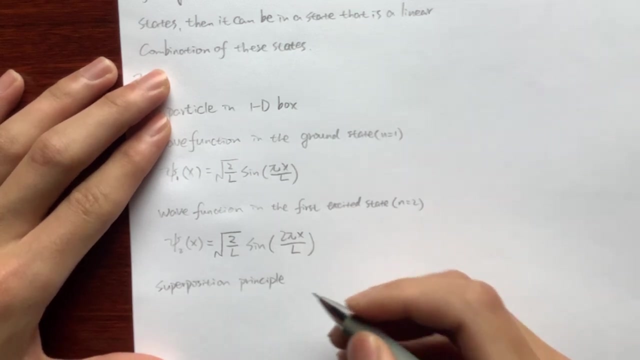 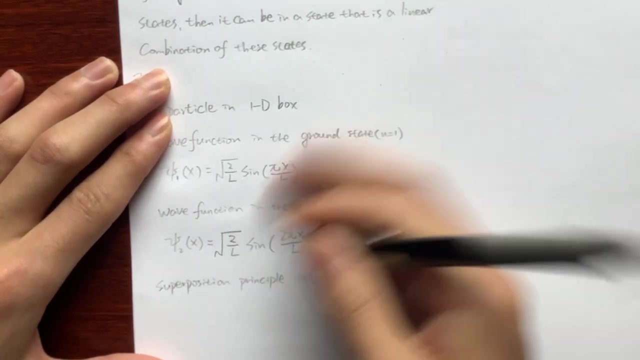 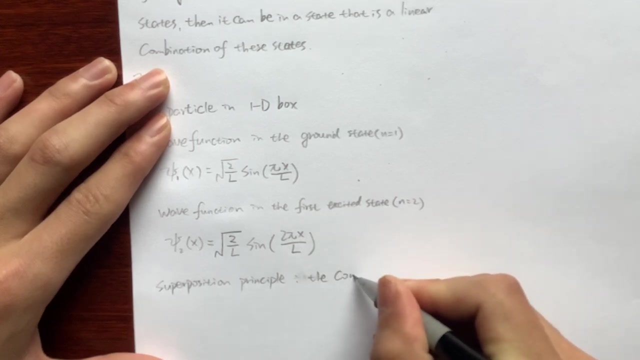 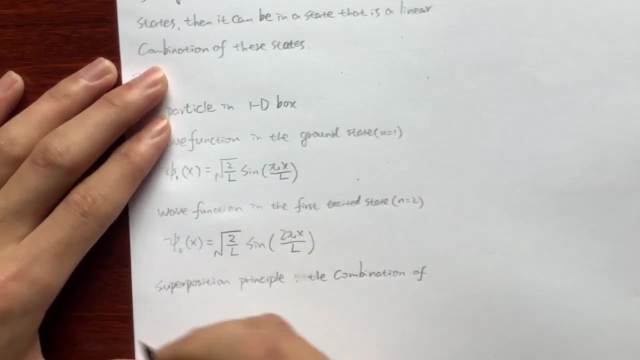 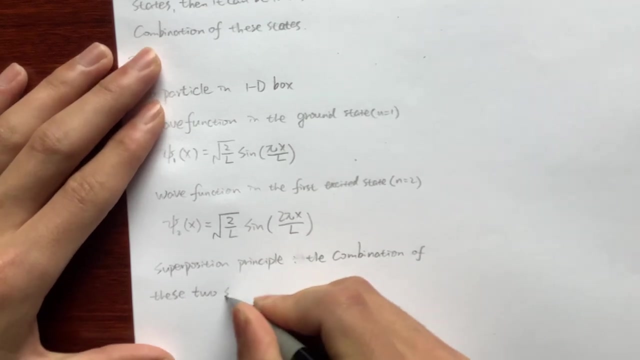 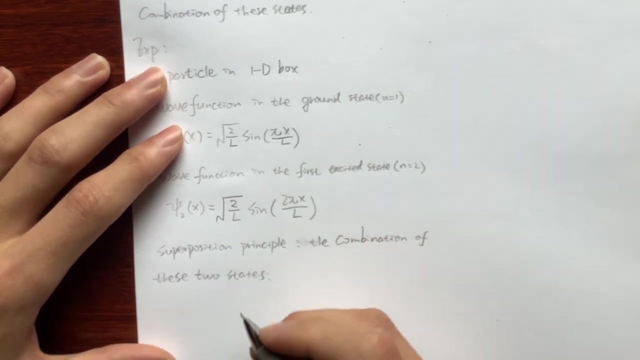 We can use the superposition principle to create a new wheel function that is a linear combination of these two states. so we apply the superposition principle, The combination of these two states. we can write it as: phi of x equals to c1, phi sub 1 of x plus c2, phi sub 2 of x. 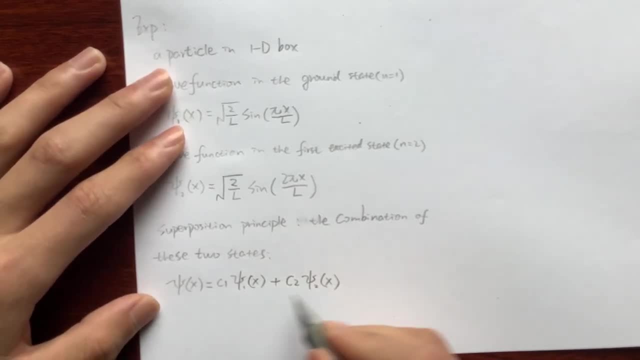 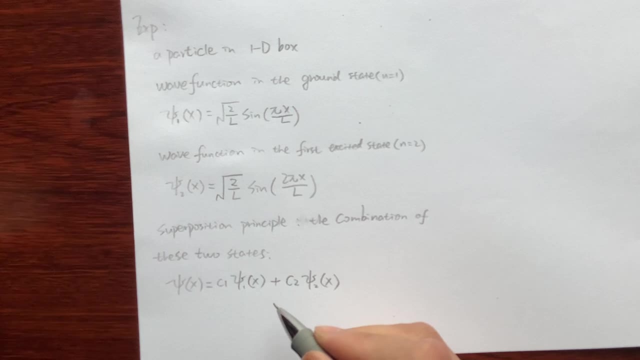 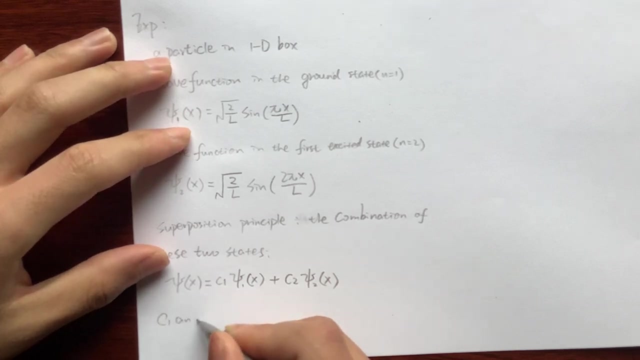 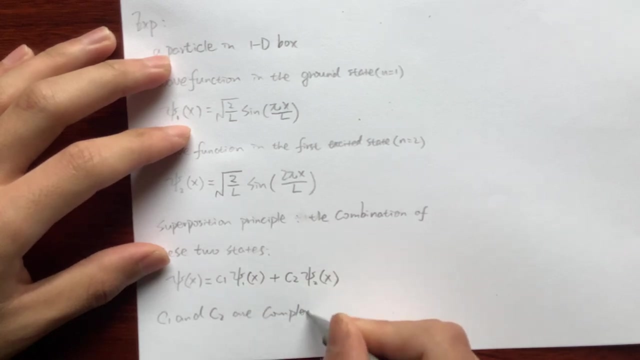 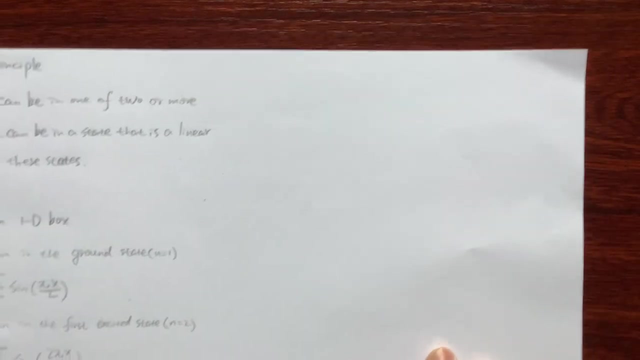 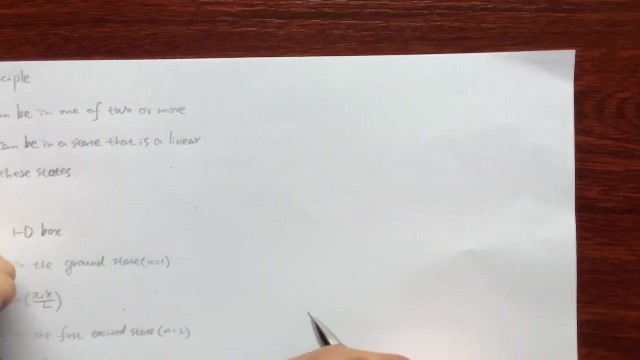 Now in here. the coefficient c1 and c2 are complex constants that determine the relative amplitudes of phi 1 and phi 2 in the superposition. The new wheel function. phi is also a stationary state, which means that density of finding the particle does not change with time. 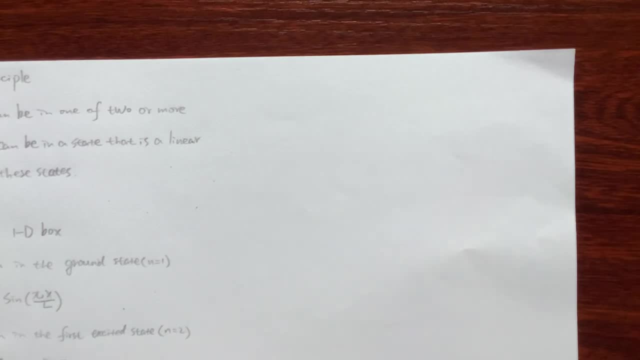 The superposition principle allows us to describe a more complex system by combining multiple stationary states. For example, if the wave function for a particle in a box can be written as a superposition of multiple stationary states each corresponding to a different energy level, this allows us to describe the behavior of the particle as its translations. 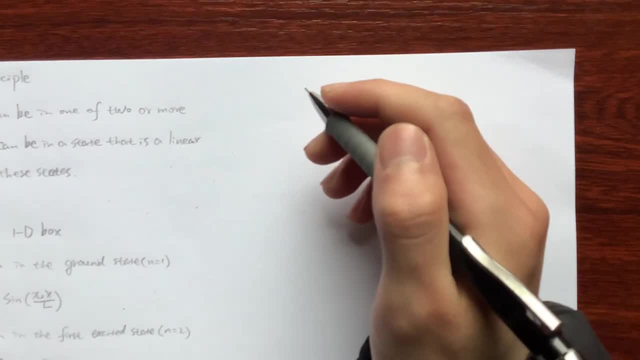 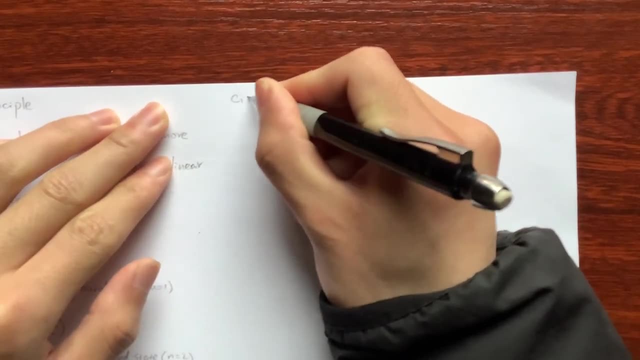 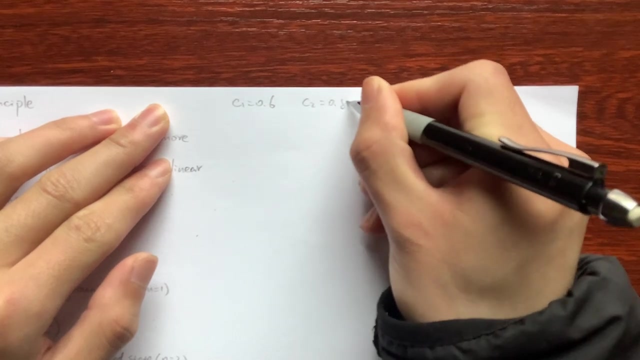 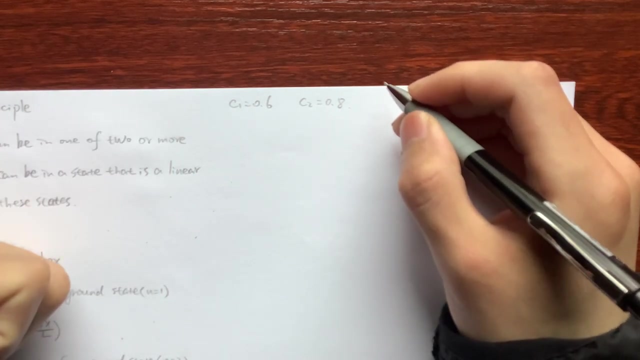 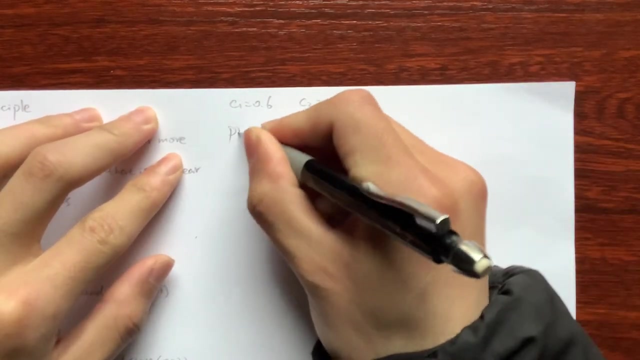 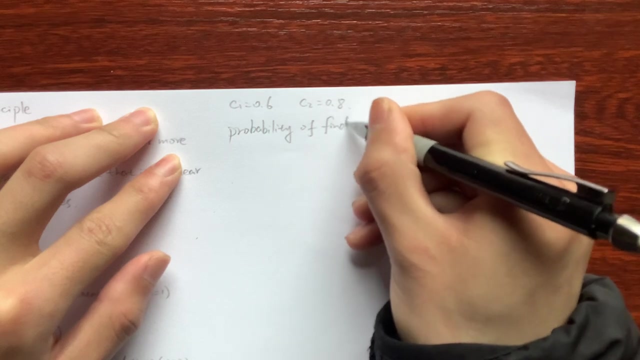 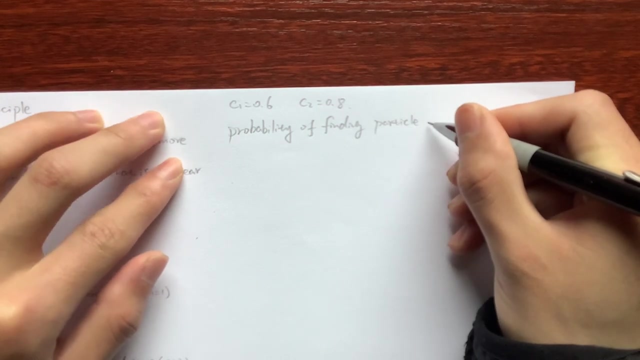 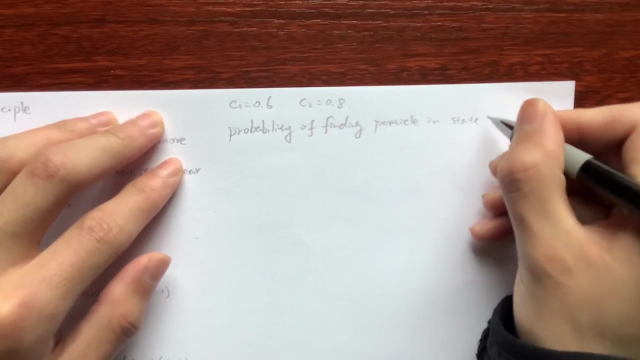 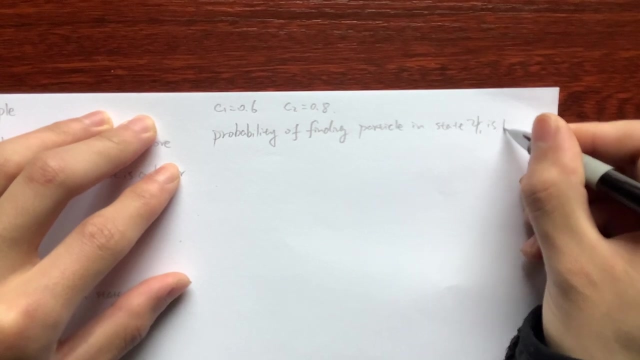 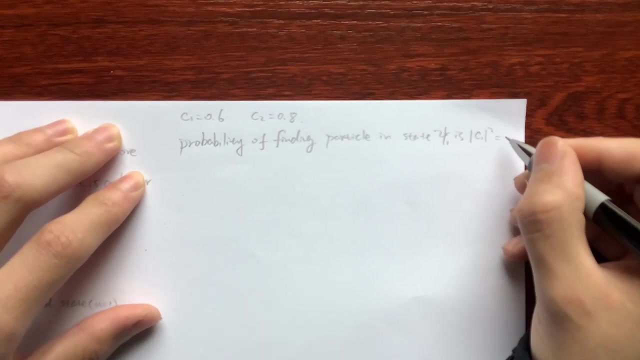 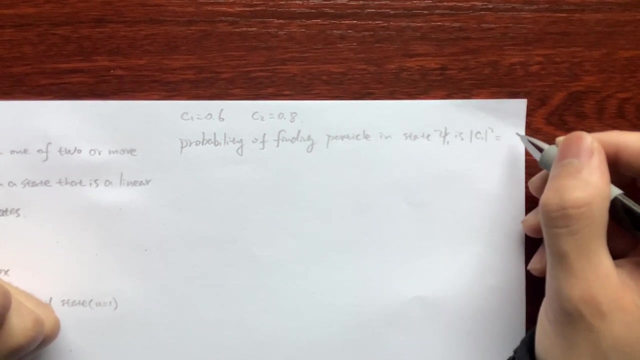 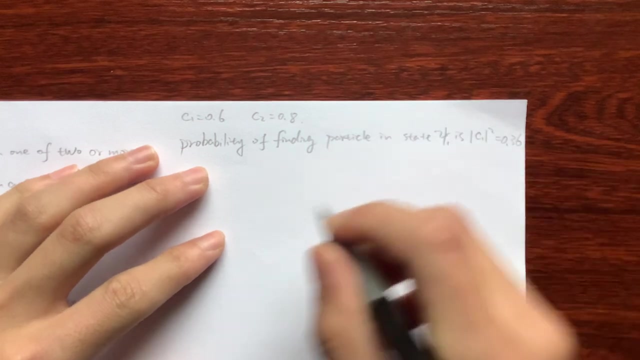 between energy levels, For example, if C1 equals 0.6 and C2 equals 0.8.. Now the probability of finding the particle in state phi1 is the absolute value of C1 squared, which is equal to 0.36..